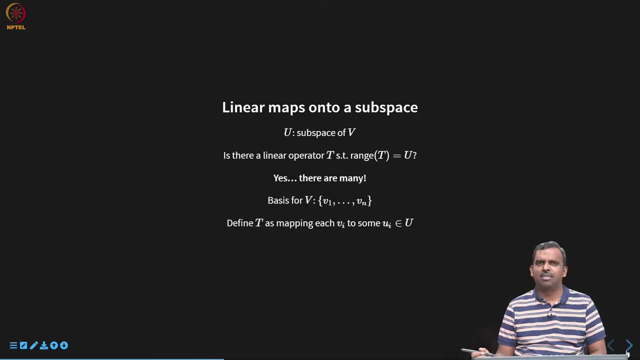 asking for something which is too much. Well, it turns out: yes, in fact, there are quite a few you can start with. So how do you specify a linear map T? you have to linear operator T. you have to look at the basis for V, any basis that you like. 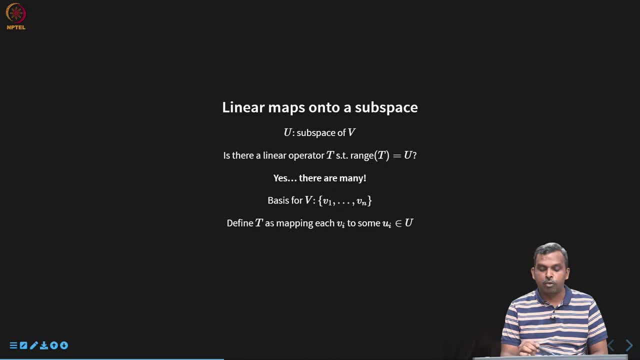 And for each Vi in the basis I have to say what T maps it into. So as long as T maps each vector here into something in u, you will always have the range being inside u. In fact, you can make it equal to u by choosing enough independent vectors inside u in this form mapping. 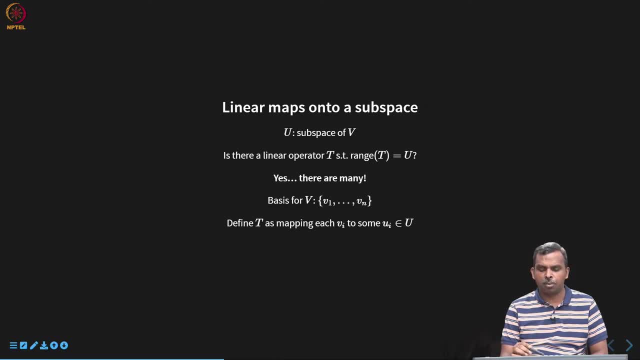 So this seems like it is easy to do, So I can make a linear operator in this fashion very easily, So I can send a vector from my vector space into the subspace of choice. So out of all these kind of choices there is one special choice which is called orthogonal. 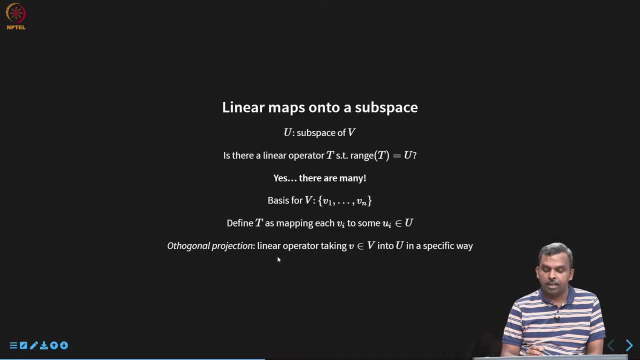 projection and it has a lot of powerful properties And it is one specific linear operator which will take any vector into the subspace u or onto the subspace u And, in a particular way, this orthogonal projection sort of way. I will describe what that is as we go along but this: 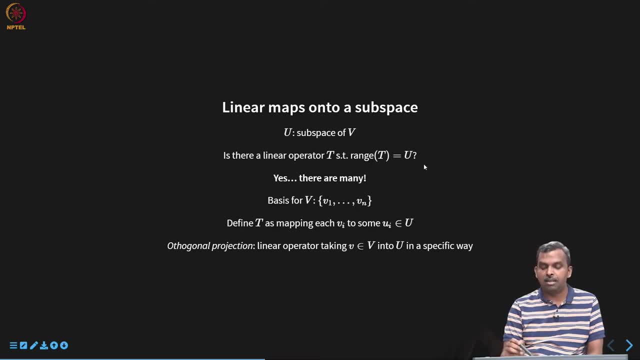 is the context, and you can keep this in mind. then also remember that there are many possible operators which can take you into a space. out of them, this orthogonal projection is a little bit special, So we will see what is special about it as we go on. 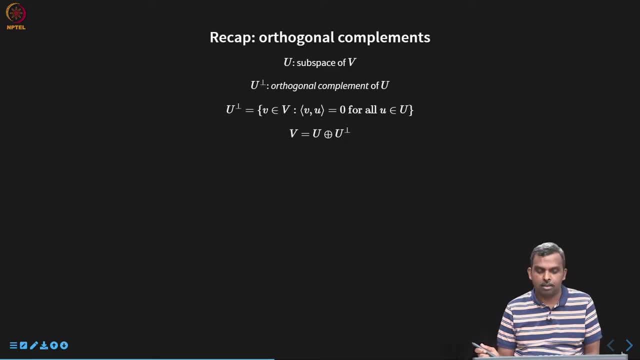 A quick recap of orthogonal complements. we saw that in a previous lecture. supposing you have a subspace of a vector space, we define the orthogonal complement as the collection of all vectors, such that the all vectors that are orthogonal to every vector in u. 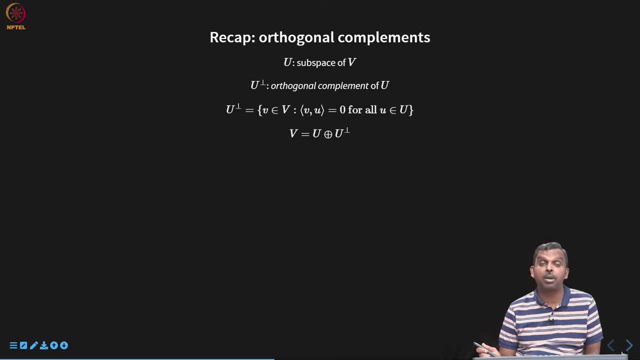 So that is how we define orthogonal. So that is how we define orthogonal, define the orthogonal complement. we saw this wonderful property that u and u perp, the orthogonal complement of u, is denoted u- perp. u and u perp have a direct sum. 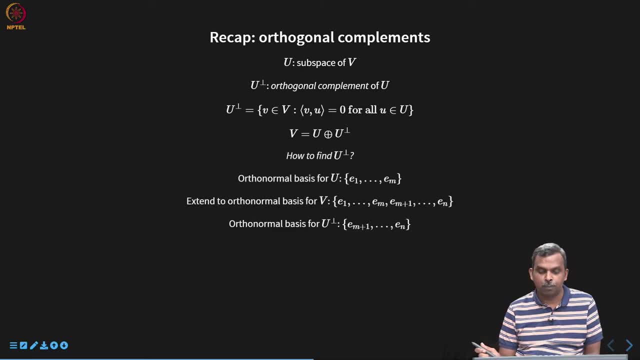 which is equal to the entire vector space V. So we saw that. And how do you find u perp? I gave you this little method here. there are other methods also, but this method is: you start with an orthonormal basis for u, you extend it into an orthonormal basis for V and then u perp is simply: 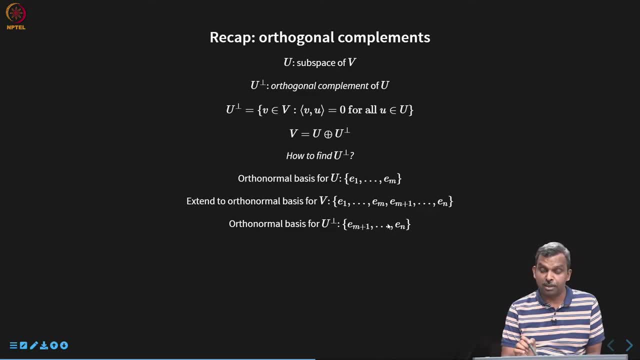 the extended vectors that you have. So the orthonormality is important here and that gives you all that you want for u perp. This is a very quick and easy way for doing constructing u perp and finding it out, And here is a little bit of a more of an explanation of what can happen here. 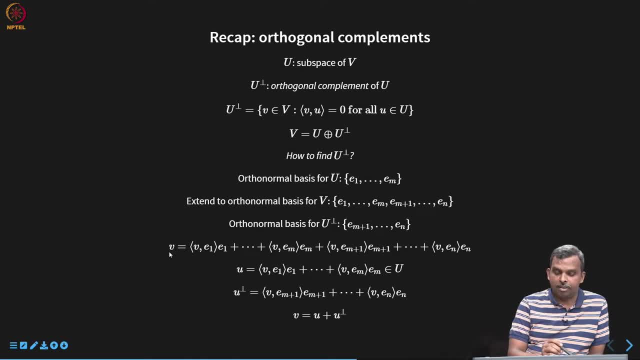 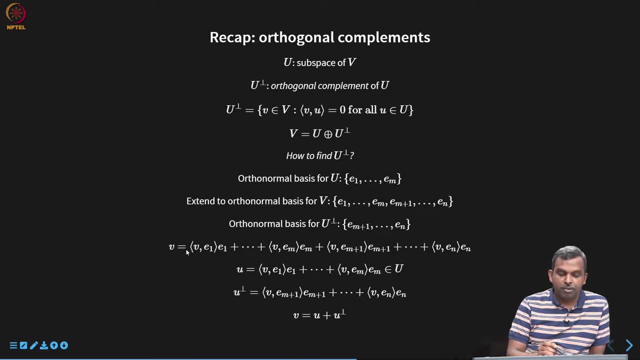 very simple formula, Because it is orthonormal. you simply have to take the inner product with respect to which it is orthonormal: V comma e1 times e1, plus dot, dot, dot entirely. So this gives you V, the entire vector V, And you can quickly identify two vectors, one in u and one in u perp. 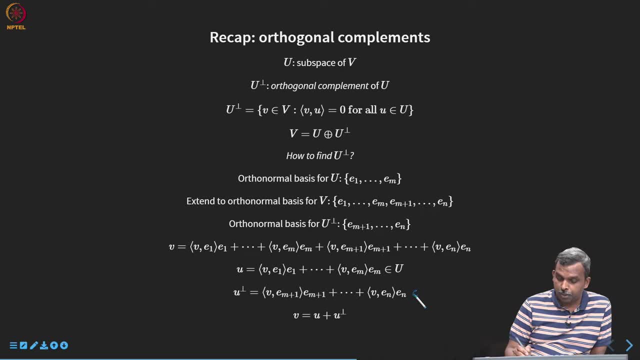 This is not mentioned here, but this belongs to u perp And the sum of these two guys, u plus u perp, is equal to V. That just directly comes from the way this orthonormal basis property behaves. Because it is orthonormal- you have this very simple expression for V- And because 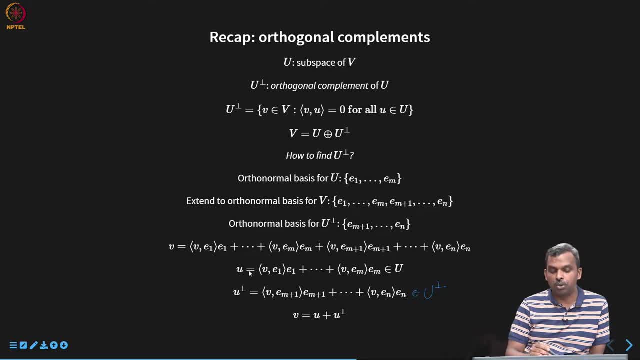 it is such a simple expression. it sort of splits into two halves, u and u perp. So you are able to identify here from the orthonormal basis extension V as the sum of two vectors, u and u perp, and they add up to V, And we also know that this is. 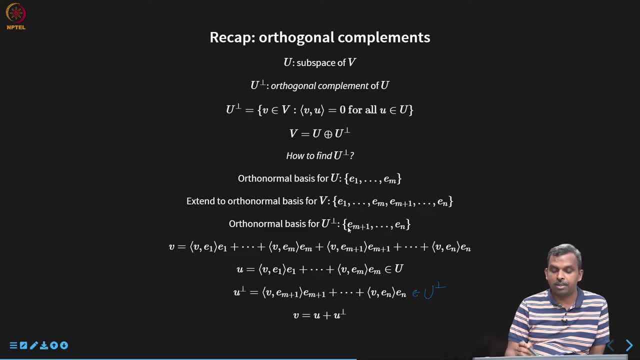 unique. This? u is unique. Irrespective of whatever orthonormal basis you pick, this? u ends up being unique. You can prove that as well. So that property we know. So let us see an example of this and sort of see how this works in practice. So here is a very simple example In class. 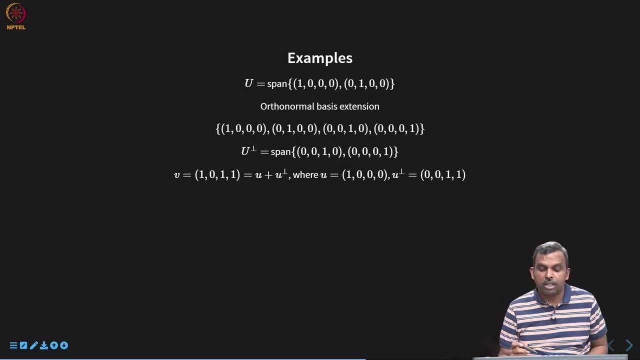 I tend to do simple examples to give you an idea of how this whole thing works. Here is a? u. I am doing this example in R4.. You can evidently see that This example is in R4.. I will start with a very simple subspace. It is spanned by these two basis vectors. 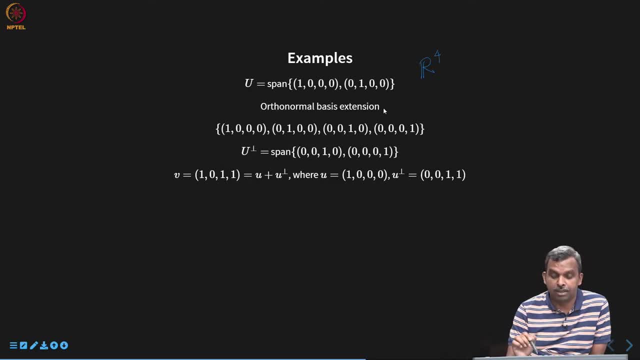 1, 0, 0, 0 and 0, 1, 0, 0.. This is clearly a basis. I will do an orthonormal basis extension. It is very easy to do. It is a standard basis. So I extend it in this fashion. So I quickly identify. 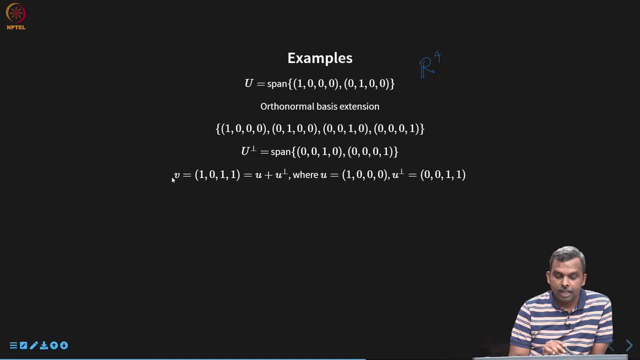 u perp as the span of the remaining two guys. That is easy, And any V. I have taken an example V here- 1, 0, 1, 1. And it can easily, quite easily be seen as u plus u perp And that is. 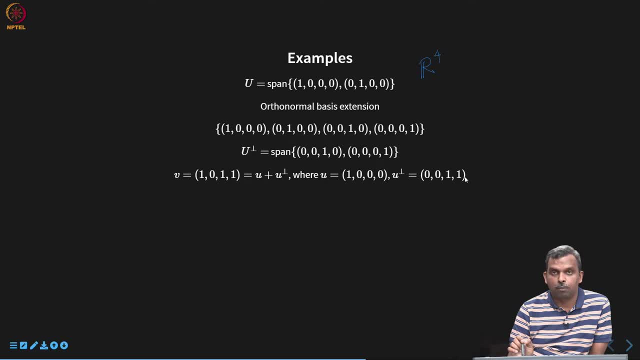 just 1, 0, 0, 0 plus 0, 0, 1, 1.. You can see that this one belongs to u perp. This one belongs to u And I mean, if you want, you can write it down in the clear way as before the inner product. 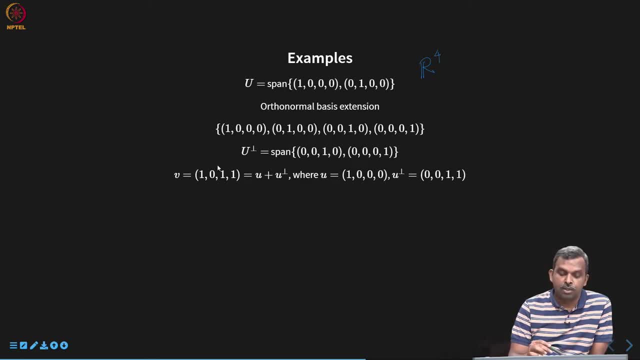 So how do you identify the coefficient? You take the inner product of these guys. So you see this is 1.. This is all 0. So you get 1, 0, 0, 0 as the u part For the u perp part. 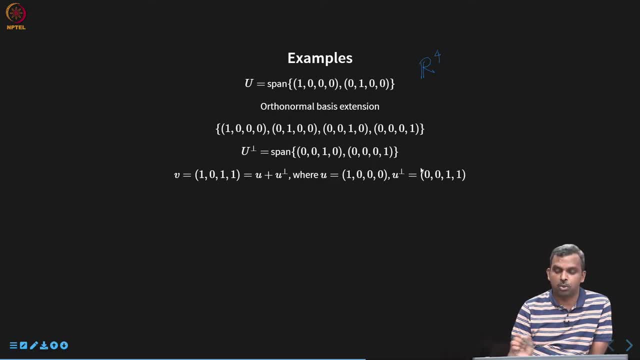 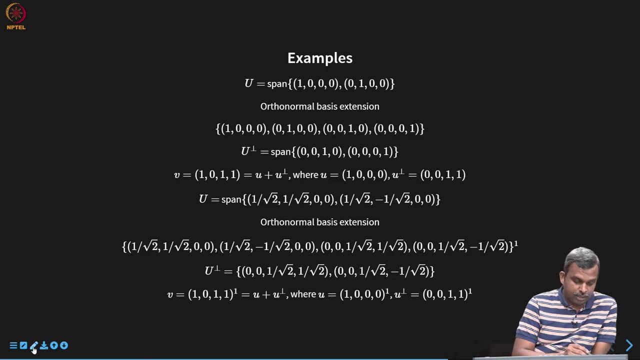 you see that first one is 0,. second one is 0,. third one is 4.. It is quite trivial to see that that formula works. So I am going to do the same thing but with a different basis. So you can see here. 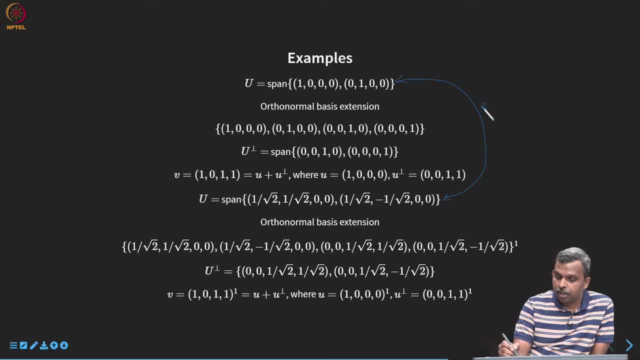 these two are equal. They are equal, but the basis is different. So different basis. It is another basis, It is also orthonormal. So this is also orthonormal. You can check that it is an orthonormal basis. 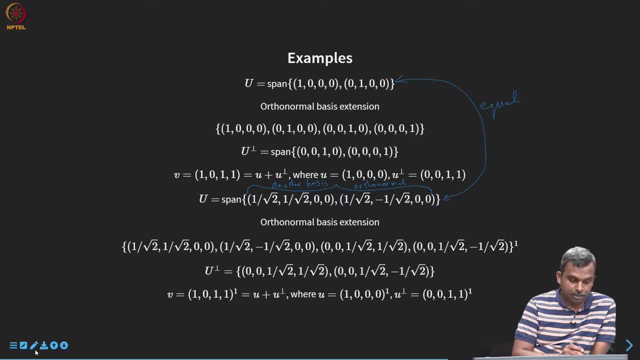 But it is not same as the standard basis. It is a different basis. So that hopefully gives you another example. I just wanted to show what happens if you take another orthonormal basis, right? So if you take this orthonormal basis, things work out like this: What if you take? 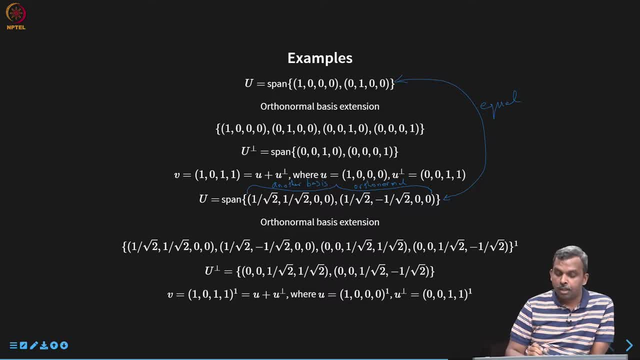 another orthonormal basis and do something else with it. Here is an orthonormal basis extension. So I have taken this guy and I have extended it to a basis for the entire vector space V. I am putting this 1 here simply to indicate that this is a different basis for me, So I have taken this. 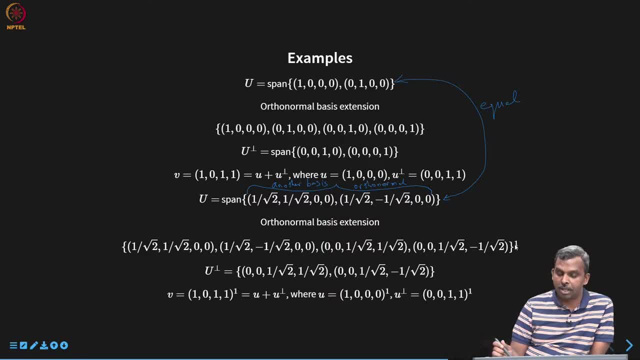 different basis, from the previous one, from the standard basis that we had. So u perp- now you can again identify- is. so you can see u perp is also the same as this. So it is the same thing, but the basis is different. So a different orthonormal basis has come. Now, if I take v, 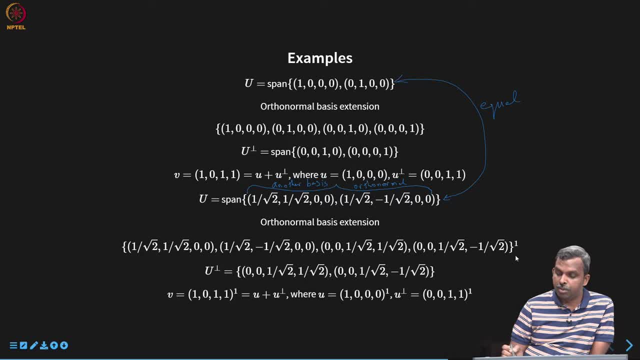 in this basis, in this new basis, I am taking a vector v. you can write it as u plus u perp, and that would again be 1, 0, 0, 0 plus 0, 0, 1, 1.. So if you want to see why that is so, 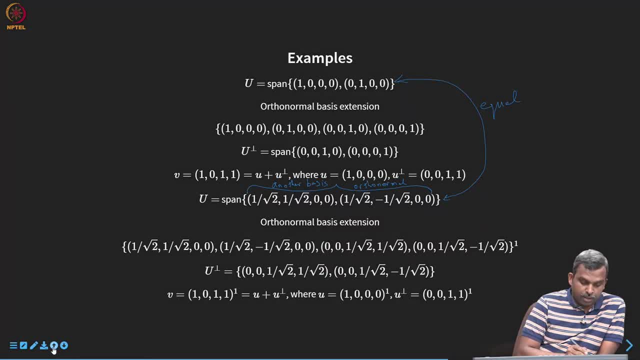 you can see. so this v, maybe I should write it down in more detail. So this v, so let us call it. I will call this e1,, this one e2,, this is e3 and this is e4,. 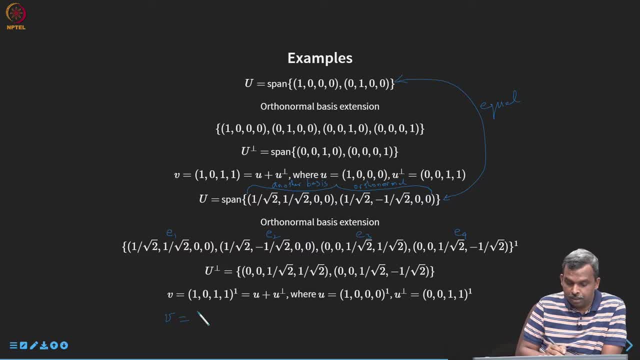 just for convenience. So what is going to be? v comma e1, the inner product of v and e1,. so that is going to be: v comma e1, the inner product of v and e1,. so that is going to be. 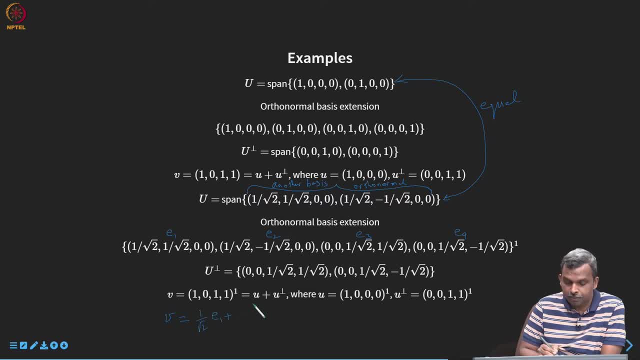 1 by root 2 times e1, plus 1 by root 2 times e2.. So I am taking the inner product here with this. No, I think did I make a mistake. Let me just strike it out. No, that is correct. I think that was correct. I do not know why I wrote that out plus. 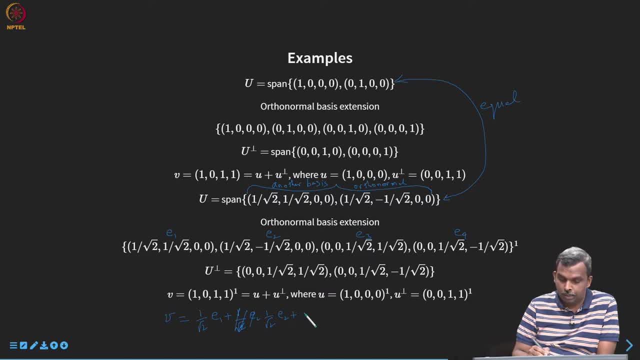 these two would again work out to something. So if you do v comma e3, that is going to be root 2 times e3, plus if I do an inner product with this, with this guy, I am going to get 0.. So this, the last one, just works out as 0. 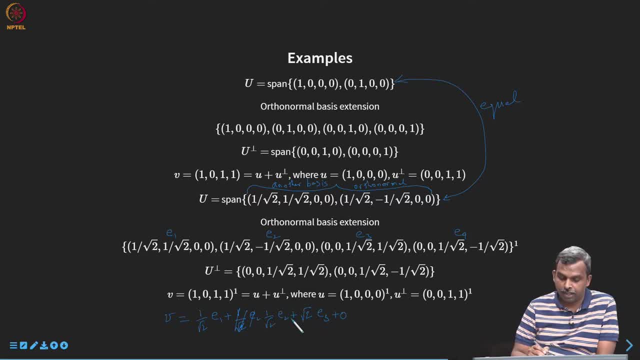 So you do not have an e4 component in this. So this is how it works out And that is v in written in this basis, if you want to write it out like that, And what is the u part? So these two together will make the u part of it. 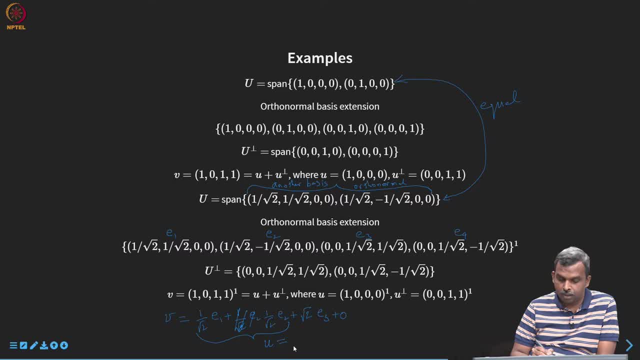 So the? u part is now 1 by root 2 e1 plus 1 by root 2 e2, and that will work out to. you can see that that will work out to 1, 0, 0, 0.. That is not in this basis, though. 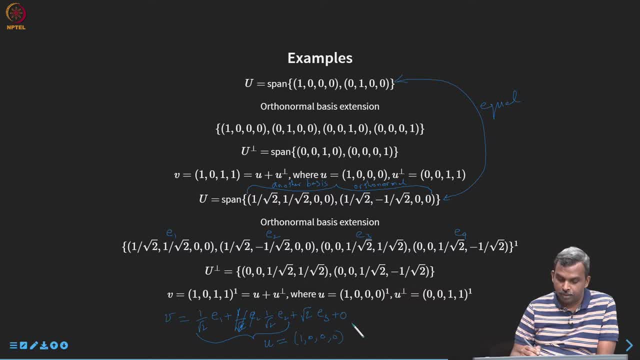 So one needs to be a bit more careful here. So it is just 1 by root 2 e1 plus 1 by root 2 e2.. So So it is just 1 by root 2 E1 plus 1 by root 2 E2.. So this is in the. I am sorry for that, I think. 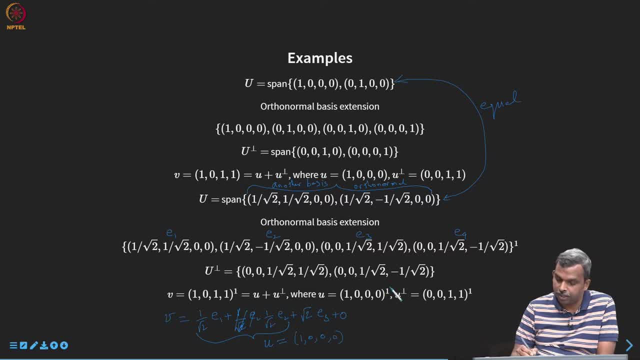 I messed this up a little bit So hopefully let me just clean this up here. So this 1 is wrong. It should not be there. It should also not be there. So this is in the original basis. So even if I pick 1, 0, 1, 1 in the new basis, you see it decomposes into U plus U perp. 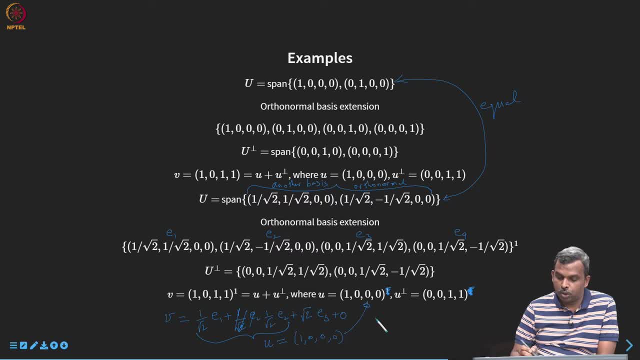 and it goes into the same U in the original basis. So of course, if you write U in the new basis it will be something else, but it goes back to the same U in the original basis. So that tells you the uniqueness of U and U, perp. 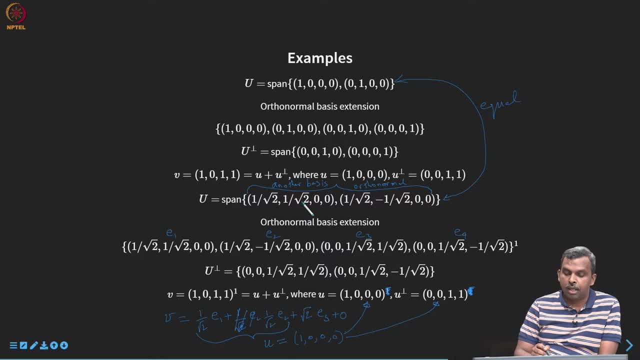 Even if you change the basis with respect to which I am doing the orthonormal basis calculation for figuring out how V decomposes into U and U perp, I will get the same vector, U and U perp. So that is clear enough to see from that point of view. 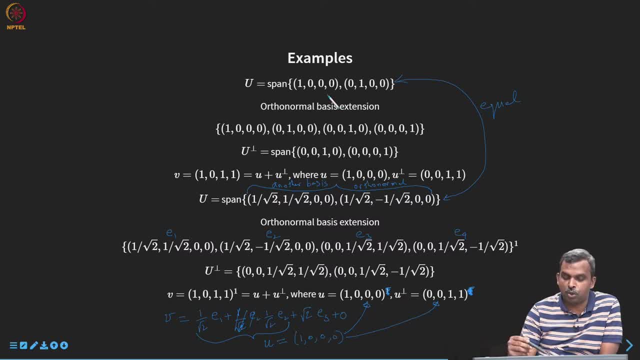 So hopefully this was a clear enough example. So basically I am showing an example of a vector, subspace U and two different basis choice for the orthonormal basis and two different orthonormal expansions. So one ends up being the standard basis. 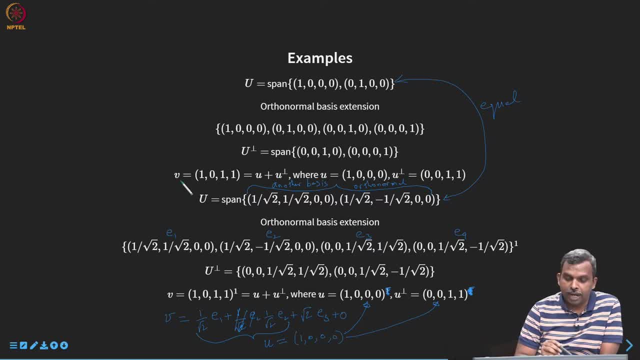 the other ends up being some other basis. And then I try to write a vector which is 1 0 1, 1. in the original basis I am writing it in terms of U plus U perp and I get 1 0 0, 0 and 0 0 1, 1.. 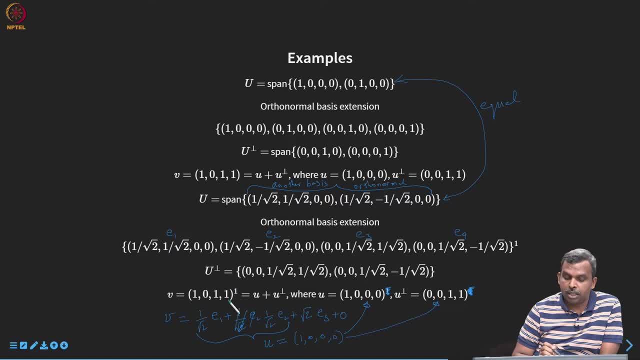 And then I take a vector which is 1 0 1, 1 in the new basis and that will end up being something else in the original basis. but because I picked 1 0, 1, 1 and then when I wrote U plus U perp, and when I saw what happens here, the U ends up being the same. 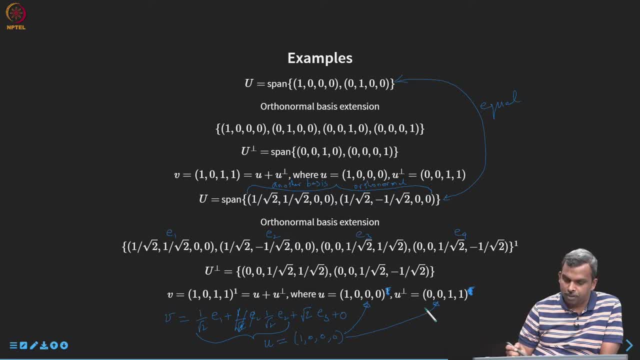 So you get the same thing there. It just stores the. it has to work out like that So that works out correctly. So u is 1 0, 1, 1 in the old basis and u- perp is again root, 2 times this. that will work out as 0 0, 1, 1 in the old basis. 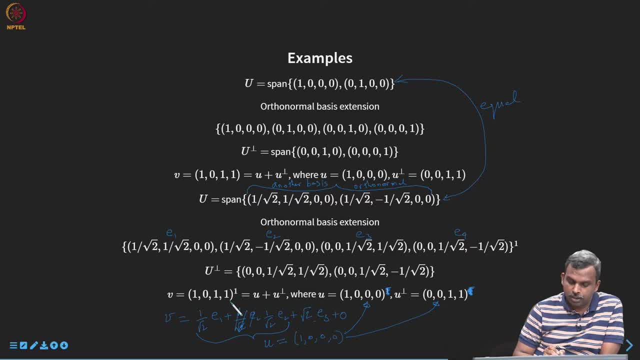 So you pick 1 0 1, 1, but this 1 0 1 1 is in the new basis. it works out in this fashion. So hopefully this example was interesting enough for you to see how the same you can pick. 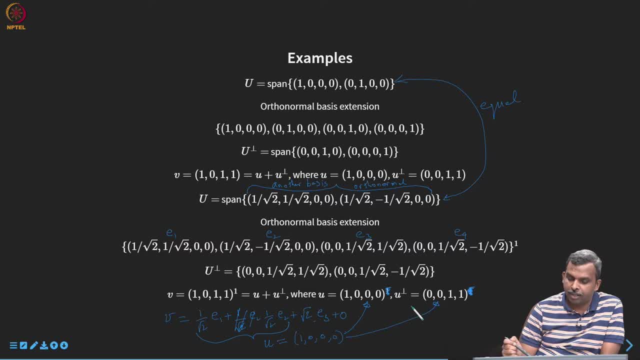 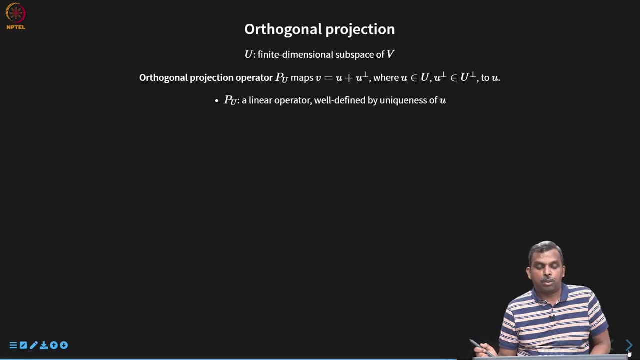 whatever basis expansion you want and you would get the result that you want here. So writing in terms of u and u, perp, is illustrated in this fashion. So let us move on to define orthogonal projection. So hopefully by now you are convinced that if you have a subspace, 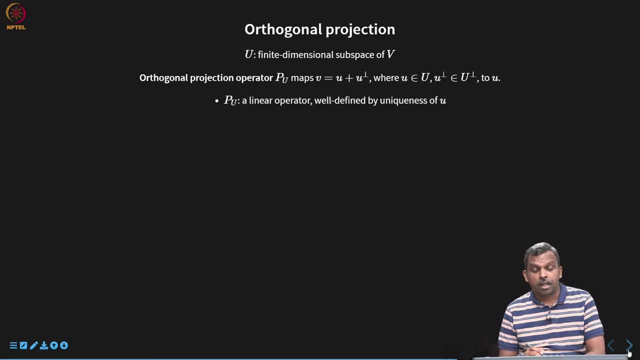 u finite dimensional subspace of a vector space, v. you can always write it as u plus u- perp. And how do you do that? You pick your favorite orthogonal basis for u, extend it to an orthogonal basis for v and then pick up only the? u part of it. you get your u. So that seems like a. 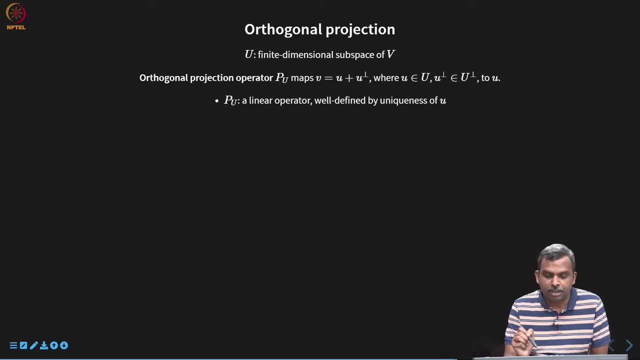 clear enough way and it is unique as per the definition here. So the orthogonal projection operator p? u basically works in this fashion. So it takes maps, a vector v to u. And what is this? u? u is obtained by the decomposition of v into u plus. 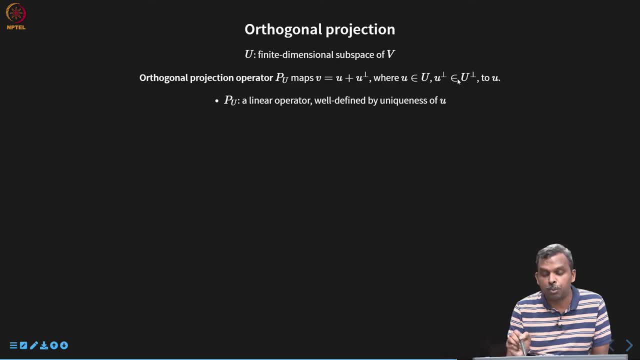 u perp and where u comes from the vector space u and u perp comes from the orthogonal complement u- perp. So clearly, this is a linear operator. you do a very cleanly linear operations and it is well defined because u is unique. whatever I mean, just because you change something. 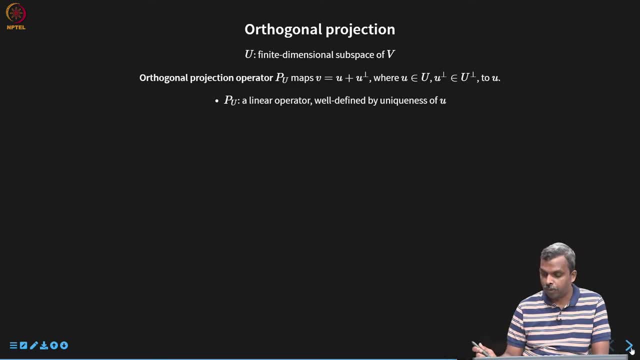 u is not going to change. u is going to be the same thing. So here is an example. So let us take a simple definition for u? u is a one-dimensional subspace, so how do you project, how do you do an orthogonal projection onto a one-dimensional subspace? u? 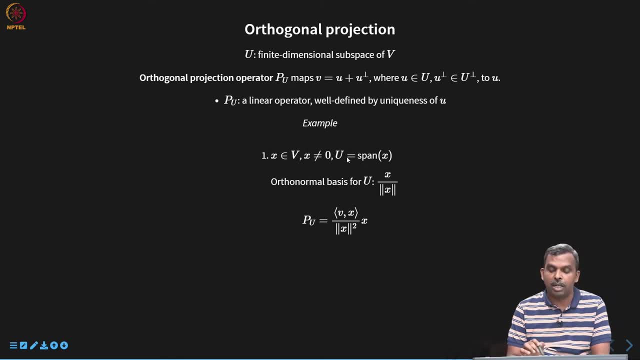 So let us take one nonzero vector and define the one-dimensional subspace as a span of that nonzero vector, x. You see quickly that the orthogonal basis for u is simply x by norm x. So this is a definition for the orthogonal basis and p? u. 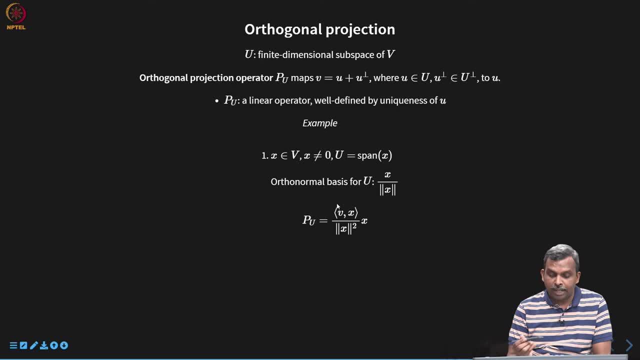 will work out as any Pu acting on any V. I am sorry, I think I am missing that here. Pu acting on any V will simply be V comma X, so V comma X divided by norm X square. So how did I get this? You can see that, So any V can be written as. so how would you? 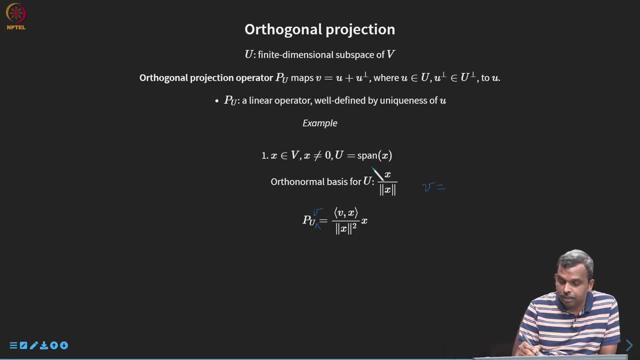 do this. So let us say we call this E1 and you extend E1, so you extend to get a basis E1, E2, so on En. So this guy gives you U all of these, give you U perp. So when you write V as V comma, E1, E1 plus dot, dot, dot, dot, dot. 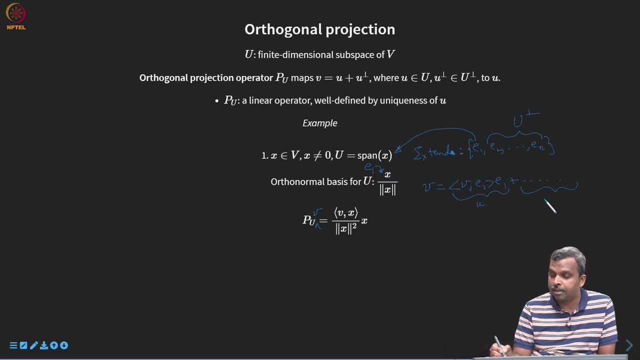 this is the projection U. this part is the U- perp. So when you project, what do you do? You write V as something that belongs to U, plus something that belongs to U perp. All that belongs to U perp. you can throw away. only this you keep, and that you can see is the same as this. 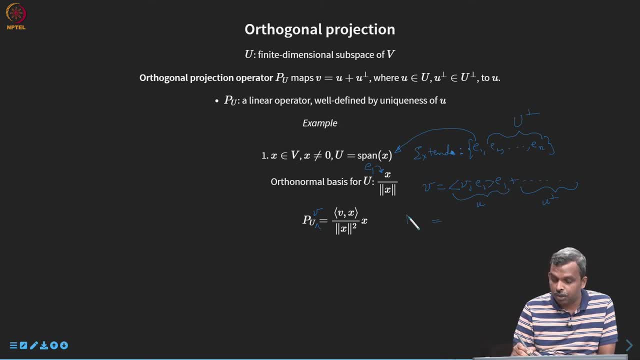 So what is this? This will work out as: so Pu times V will work out as V comma X by norm X times E1.. Again, which is X by norm X, and you can see that is the same as this. So 1 by mod X will come, norm X will come out. so you will get V comma X by norm X square times X. 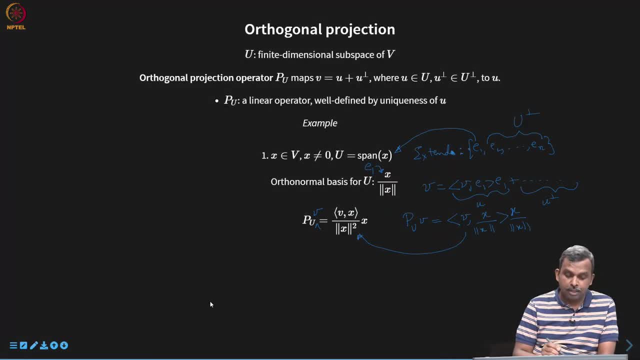 So this is how you do projection onto a one-dimensional subspace. So it just works exactly by that basis: extension argument. So you can also do for a two-dimensional subspace. you take linearly independent X and Y and then define U as the span of X- Y, you do. 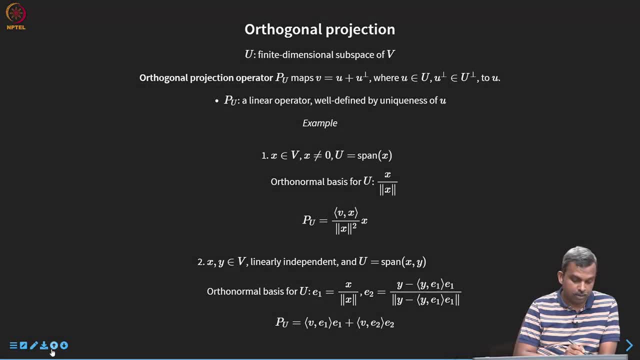 orthonormal basis. This is just Gramb-Schmidt. So this is just the Gramb-Schmidt, followed on two Gramb-Schmidt done on two vectors. how to do this? So Pu times V, I am missing the V again. 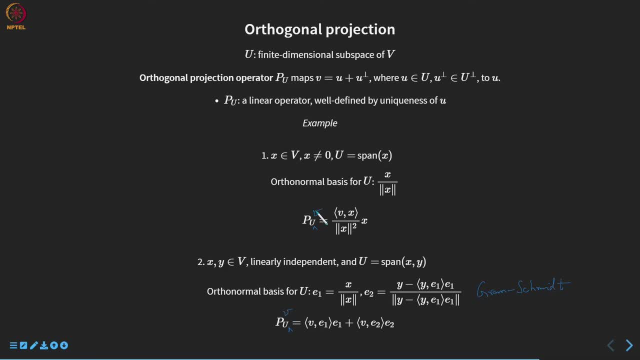 apologies for that. So Pu times V is simply V comma E1, E1 plus V comma E2, E2.. So that is it. So in this case this is the same as the span of X. So in this case, this is the span of White. 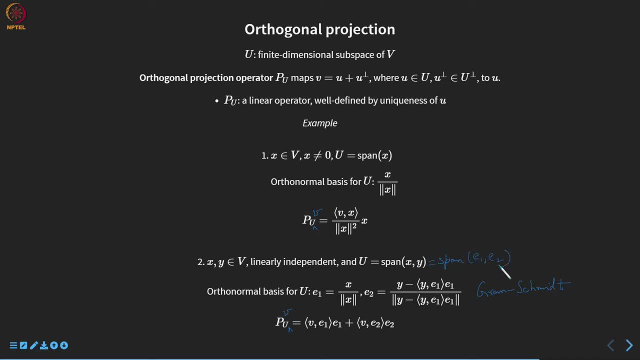 same as the span of E1 comma E2 and simply the projection on V is simply V comma E1, E1 plus V comma E2, E2.. So it is easy enough to see. So you find an orthonormal basis, any orthonormal. 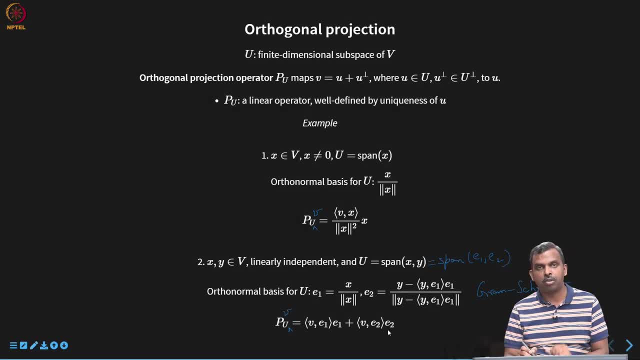 basis that you want for your subspace U and simply do this formula V, comma. each of these things times the basis that gives you the orthogonal projection of a vector V onto the subspace U. And it does not matter what subspace you pick, what basis you pick here. 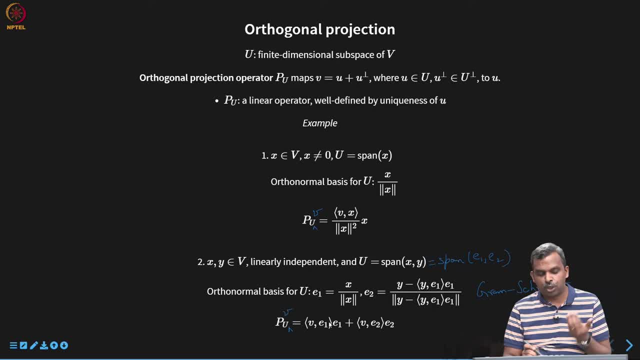 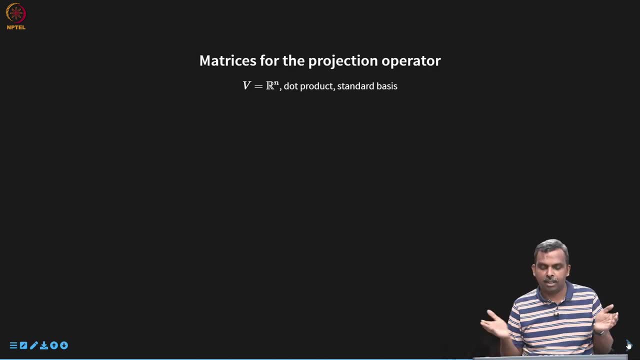 any orthonormal basis you pick, you will get the same projection operator, Pu. So that is something that we saw. So let us look at matrices for the projection operator. So we see that projection is a linear operation and we have an operator for it. We have sort of a. 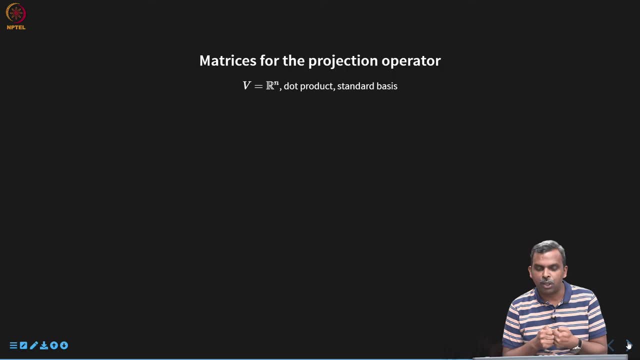 description for it. in terms of inner product. that is not too bad, it is pretty good. But let us see if we can get a matrix. So for that I will specialize to this simple example of V being Rn. I will look at dot. 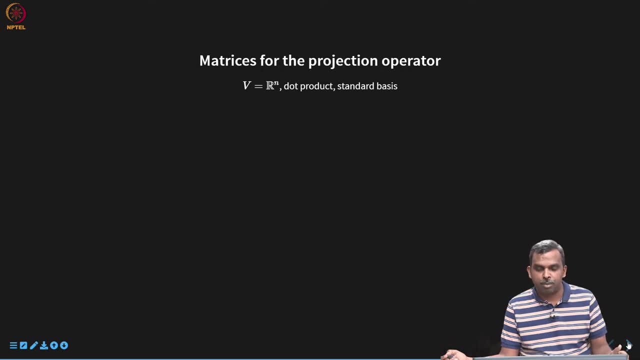 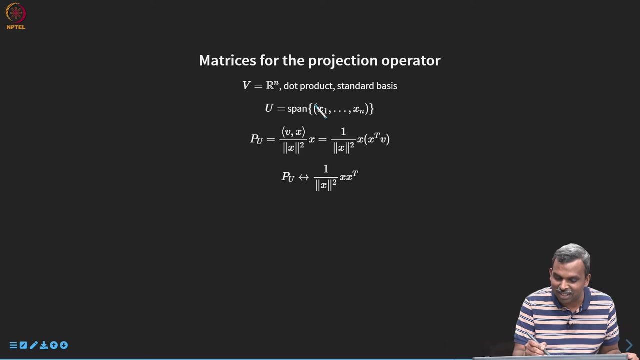 product as the inner product and the standard basis as the basis of choice. So let us do all this. And here is a? U. I have taken the vector space U to be a one-dimensional subspace. So this whole thing is a vector. do not think of this as n vectors. this whole thing is one vector. 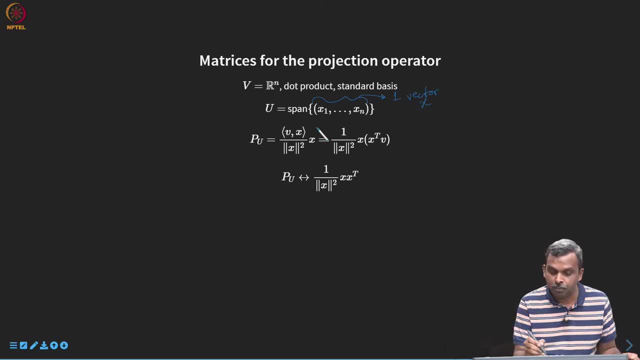 just one vector X. So think of it as one vector X And I know my projection operator acting on V. once again, sorry about that, I am missing this Pu V. here is simply V comma X divided by norm, X square times X. So that would be. I can rewrite this See. notice this see. 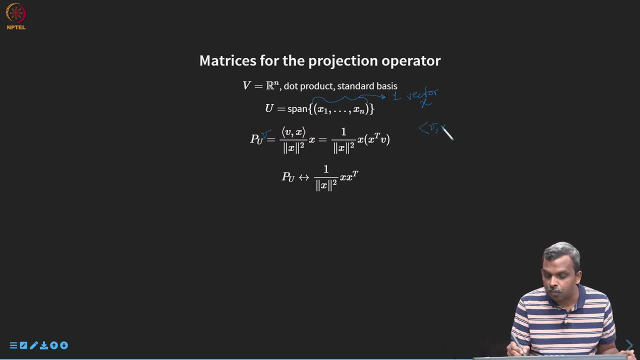 in Rn, for instance V comma X. you can write in matrix form. if you have the coordinate expansions, you can write it as X transpose V. you can also write it as V transpose X. both of these are the same. So this is. 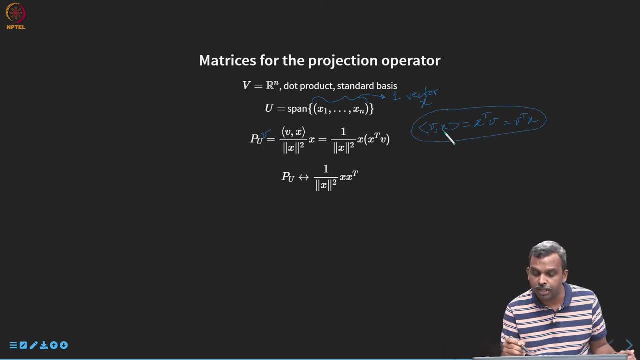 something that I did not maybe emphasize too much when we discussed inner product In Rn, where the inner product is simply, I know, the dot product, V, comma, X. inner product is the same as X transpose V. you can also write it as V transpose X. both of these are the same. important to understand this. 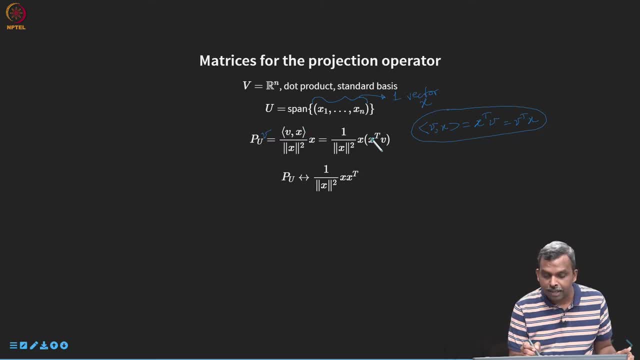 So once I know this, this inner product V, comma X, I can write it as X transpose V. So there is a reason why I am writing it as X transpose V. if you write it as V transpose X, it will not work out quite so nicely. So this is: X into X, transpose into V. I can write: 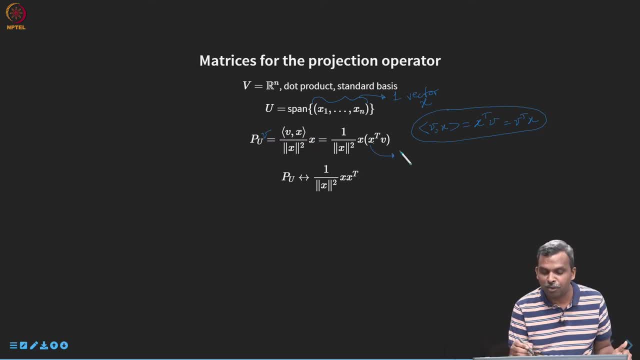 this as so. this is all scalars, so I can push it to this side if I want. So I simply I get that X into X. transpose into V is the same as X times X transpose times V. See remember, X is a column vector. I am thinking of X as a column vector. 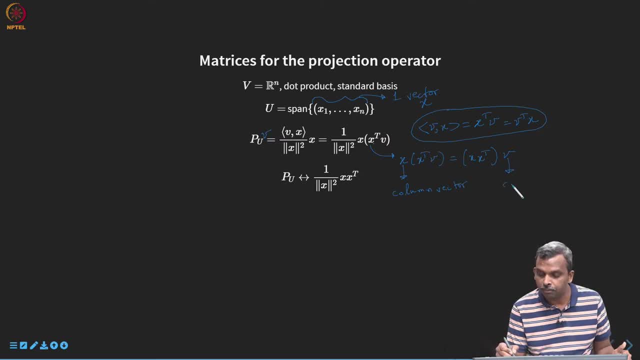 so X transpose will become a row vector and V also as a column vector. So I don't have to write these next four corners here, I can just wrote the callers in the next four corners here and close it in a row hand vector. So X times X transpose will be a matrix, N cross N matrix and then V will multiply on the. 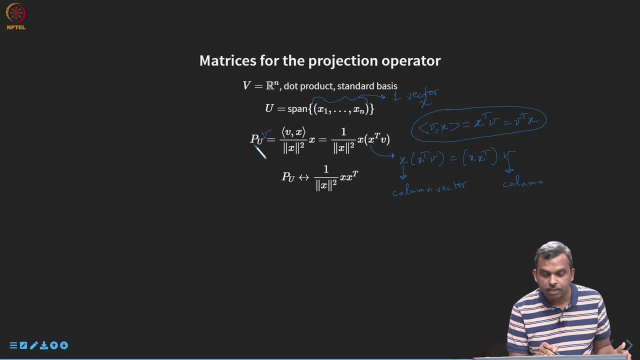 right, So this P? u, which is the operator, can be identified now with 1 by norm, X square, X, X transpose, is it So? this is the crucial thing. This is a matrix of a projection operator, So it will look like this. You can see. it is quite simple. It is X. 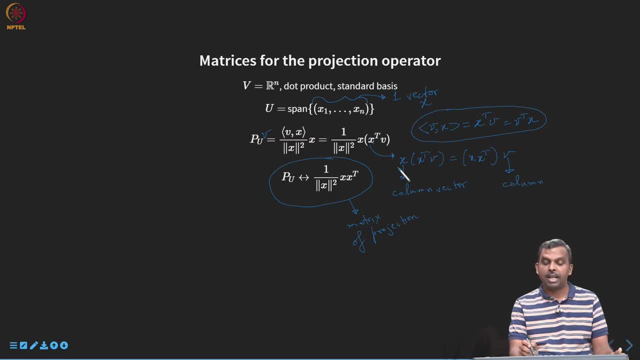 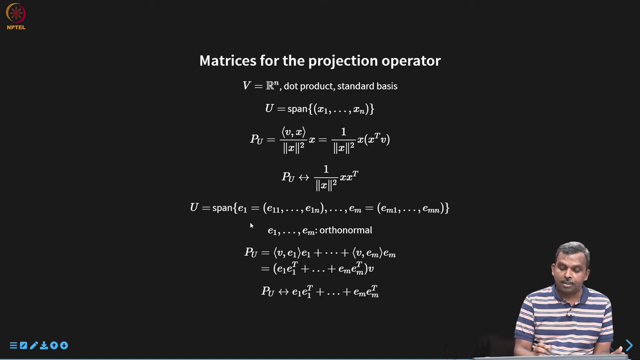 X transpose. So it is a rank 1, N by N matrix, then multiplied by 1 by norm X square. So this becomes the projection operator. So you can generalize this. It is not very difficult to generalize this. So you find an orthonormal basis for your subspace. 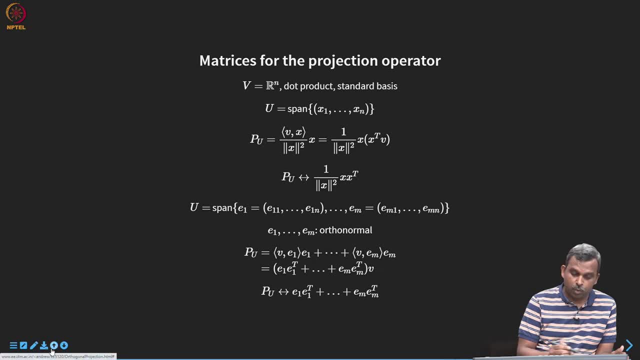 u onto which you want to project, And then if you want to do P? u times V- I am forgetting this in every single slide here- If you want to do P? u times V, you should do it here also. That will be simply V, comma, E1 times E1, and so on. So this we know. 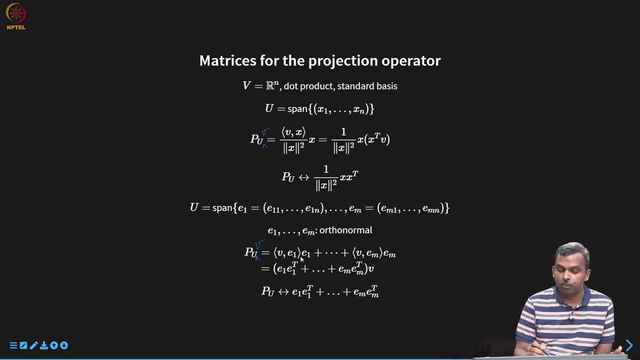 You can pick any orthonormal basis that you like for u And P. u times V simply becomes this: So now every V comma, E1, I can write as E1, transpose V And then, if you do that, you can pull the V transpose. you can pull the V transpose. you can pull the V transpose. you can pull the V. 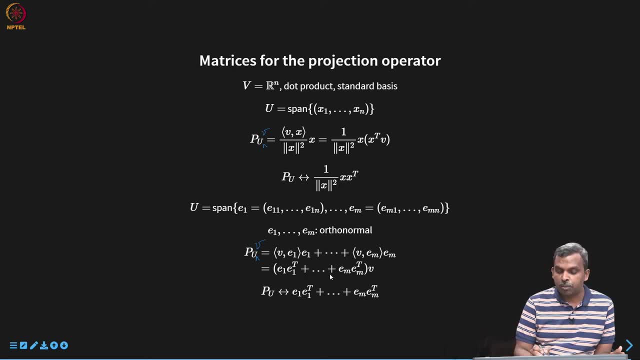 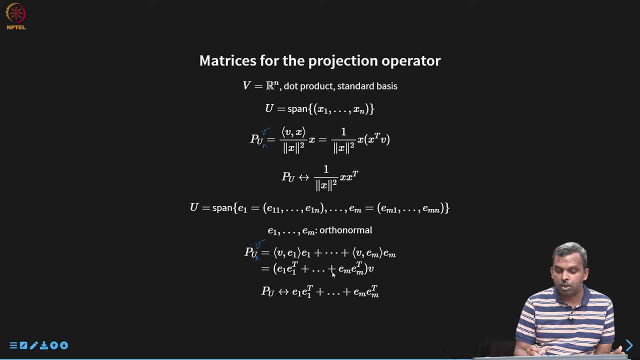 this P? u with this matrix that you got, E1, E1 transpose, plus dot dot dot, em, em transpose. So this is your n? cross n matrix which represents projection to onto the subspace. u, which is spanned by an orthonormal basis, E1 through em. So you see how. 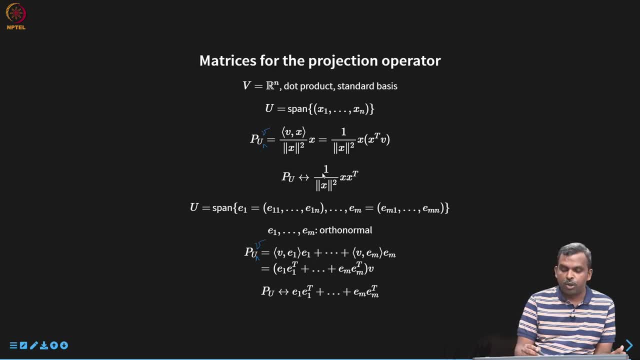 this is coming through, So this probably gives you a good idea. You do not need the one binomic square, because all these Ei's are already orthonormal, So they do not enter the picture, So it just becomes. 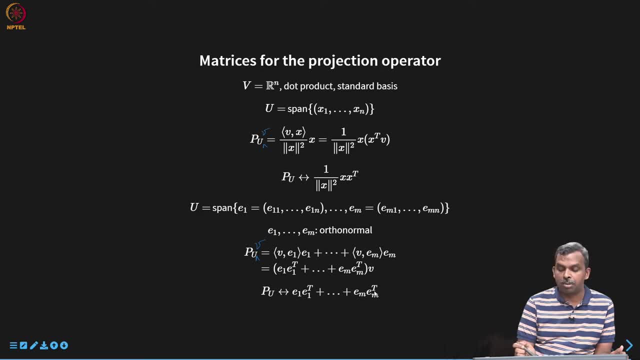 something like so. So projection onto a subspace. when you have an orthonormal basis, finding the matrix is very easy. You can repeat it quite easily for the complex case also. So instead of being X transpose V, it will be X bar transpose V. 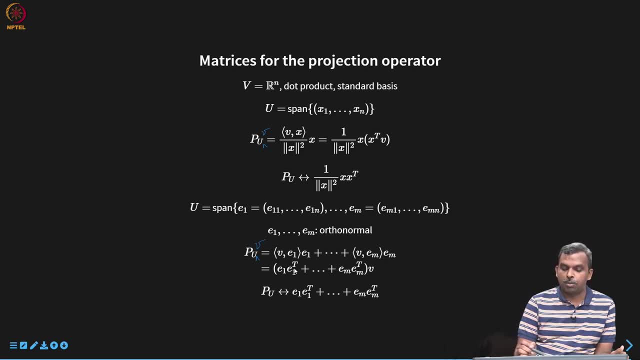 or something like that, And then that would so, instead of E1- E1 transpose, it will be E1 bar, E1 transpose, or something like that. So you should take the constant conjugate in one of these things and you will get what you want. So, finding the matrix for the 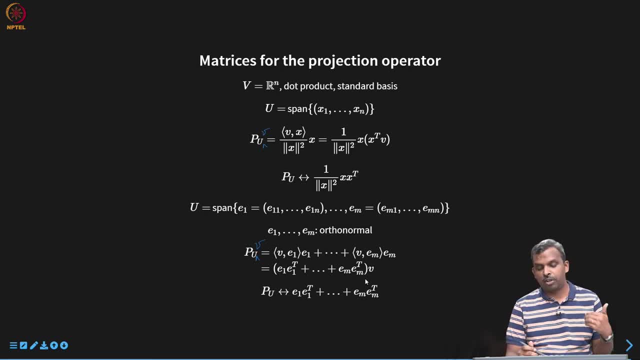 projection operator is also very easy. So you have to get familiar with projection. It seems like very easy thing to think of, It is not very complicated, but we will use some of these properties in some non-trivial way in going forward. So here are some properties quick. 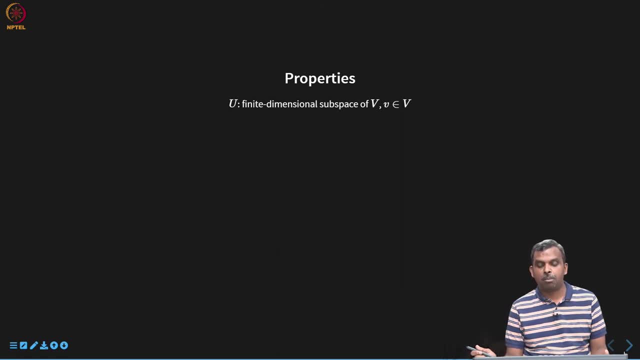 properties. one can very easily derive from the definitions I made so far, Supposing you start start with a finite dimensional subspace of V and V is some vector in the vector space. Here are a few properties, quick properties you can easily write down. If the projection operator 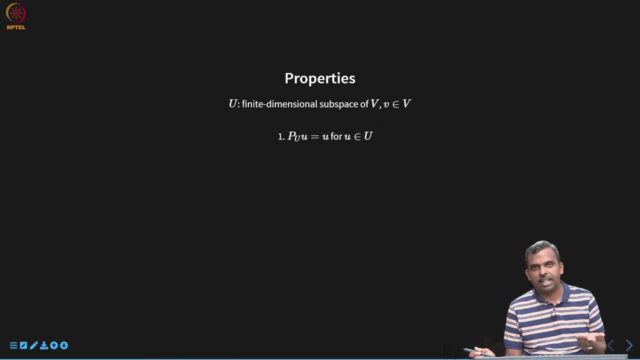 operates on a vector that is already inside U. you will not get anything different. In fact you will get exactly U. So, on the operate on the inside the subspace U, the projection operator is identity. So that is nice to know. Outside, what does it do? It makes it 0.. As an outside, 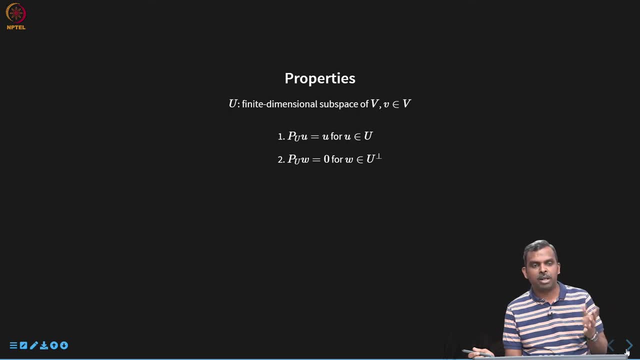 in the complement, it makes it 0. And there is also many various vectors which are outside U and which are not in the complement also. So you will have U plus U bar where U perp. then something else interesting would happen. So, but this is the story as far as how the 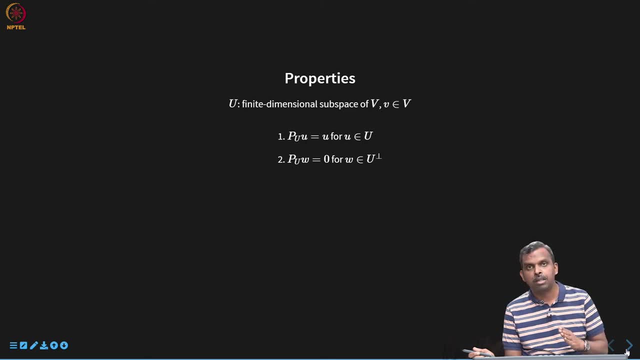 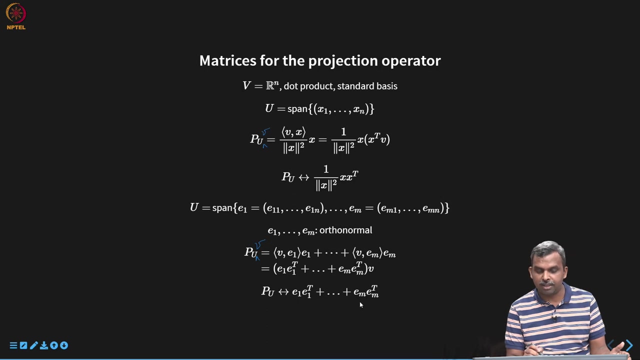 projection operator. if you restrict it to either U or U perp, how does it behave? On U, it becomes identity. On U perp it becomes 0.. So that is it sort of correlates with this description I have for the matrix. If you think about what this matrix is, you will see that. 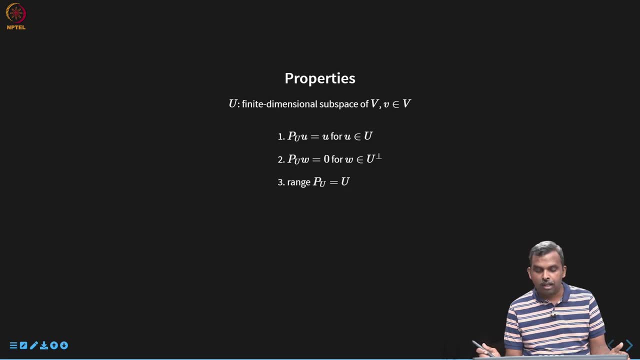 correlates very well. Range of PU is U itself. Null space of PU is U perp. These are all easy consequences And if you do V minus PUV, you get something which is in U perp. So that is also very clear from the way we defined how orthogonal projection works. If you do V minus PUV, that 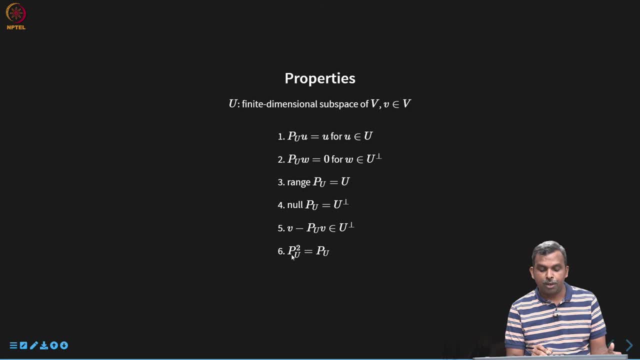 belongs to U perp. And if you do PU squared, you get PU itself. So whatever vector you have, if you square it you get the same thing as PU. So just think about it. If you repeatedly apply projection, you apply projection once you got to some point that is already inside you. If you 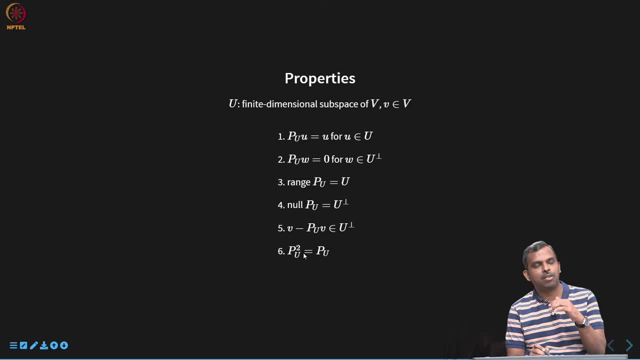 apply projection again. it is not going to change, it remains the same. So it is enough if you apply it once. So it is sort of: PU squared is a strange matrix or a strange operator. It is different, So it is not going to change. So it is enough if you apply it once. So it is sort of. 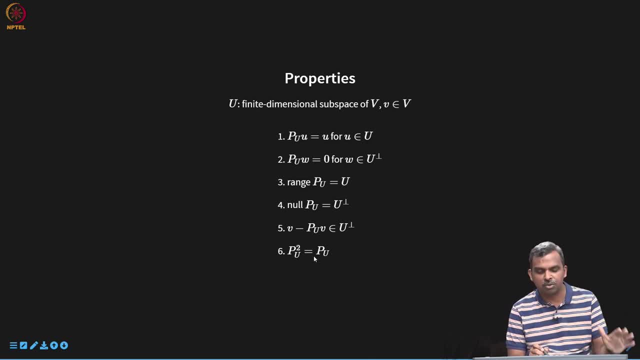 a new. you cannot repeat it The second time. you repeat it does not do anything new, It just gives you the same thing. And here is an interesting result: that norm of PUV, the norm of the projection, is lesser than the original vector, So you lose some magnitude. 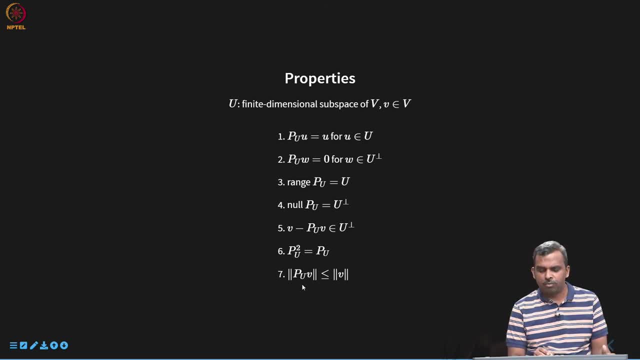 when you project to a smaller subspace- And there are proofs for all of this, And this one is a direct consequence of the Pythagorean identity- So V splits into its projection on U plus something which is orthogonal to that. So when you have two, 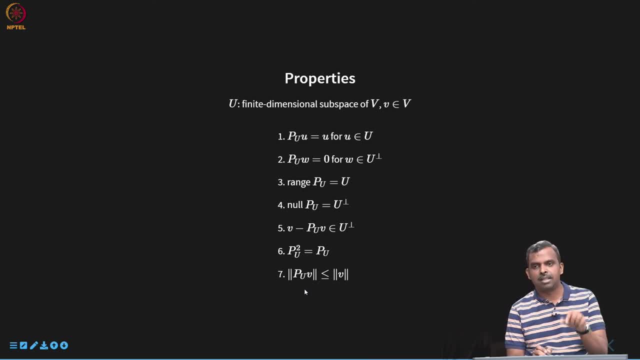 orthogonal things adding to give you a vector. the norm is the sum of those two. So since you are losing something definite, you will get the norm for the projection being lesser than this. So these are all properties. So projection is an interesting operation that you do on a vector. 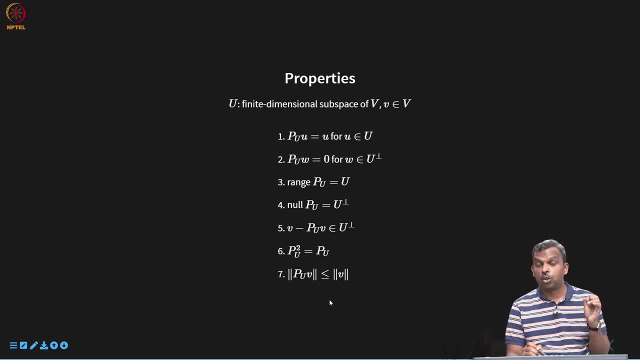 You can project onto a subspace of your choice. Orthonormal basis plays a big role in the projection And projection is a very interesting operator in the sense you do it once you go to the subspace and after that it does not.